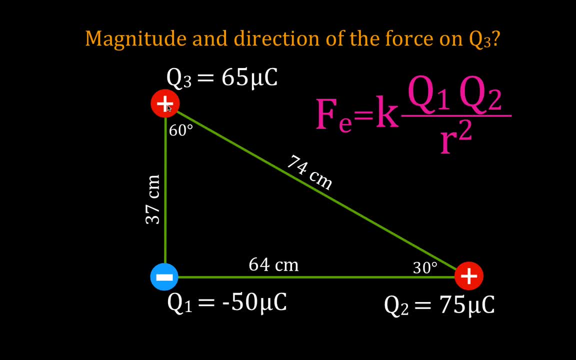 to figure out whether they're going to repel or attract each other. So first of all, we'll do Q1, since Q1 is number one, The force on three from one. this is a negative, this is a positive opposite charges attract each other. So therefore, the 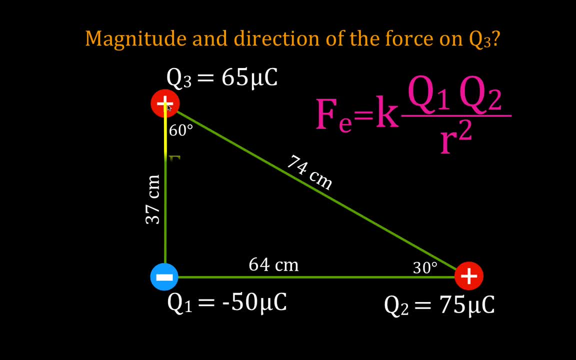 force on Q3 from Q1 is going to point in the negative y direction or point in that direction. Okay, that's just the direction, That's not the magnitude. First we're going to do the directions of each and then we're going to get the magnitudes and we have to add all that. 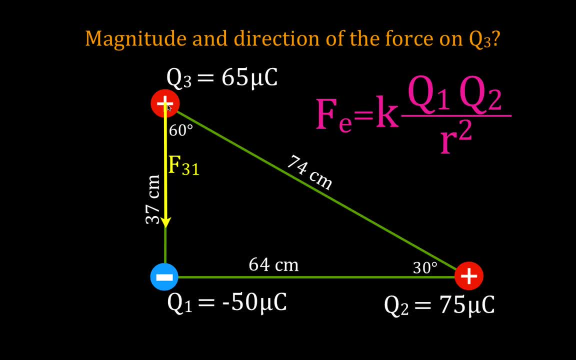 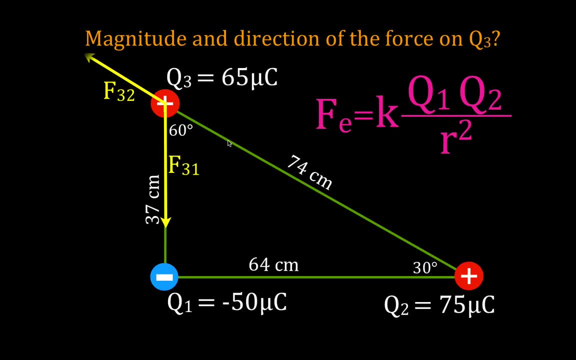 other. So Q2 is going to repel Q3 along this line. So this is the direction of the force on three from two. I didn't worry too much about how long I drew the arrows. All I really want to know is the direction when we think about and we calculate the magnitude, and then we can talk. 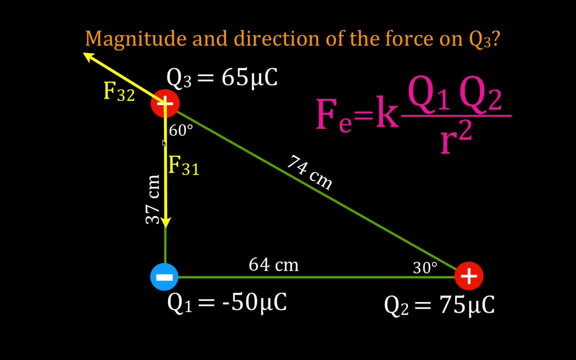 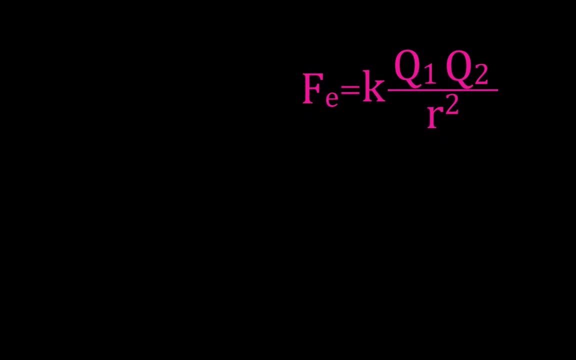 about the length of the arrows or the length of the vector, force vectors. Okay, so this is the force on three from one. This is the force on three from two. Now, in the next slide, we're going to actually calculate the magnitude of the force. Here's our diagram, Here's our 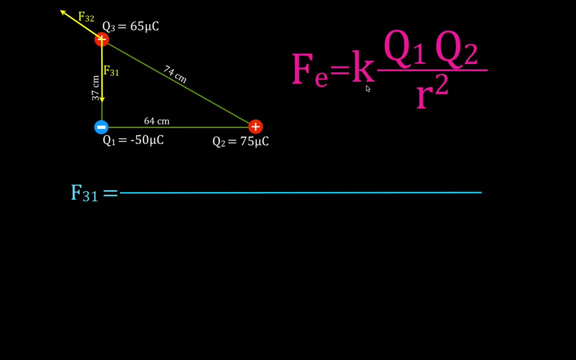 forces using Coulomb's law. We're just going to apply Coulomb's law. It's straightforward. First we'll do the force on three from one KQQR squared. Okay, Q is Coulomb's constant nine times seven, nine newton meters squared. Coulomb's squared Q1 is 65 microcoulombs. We. 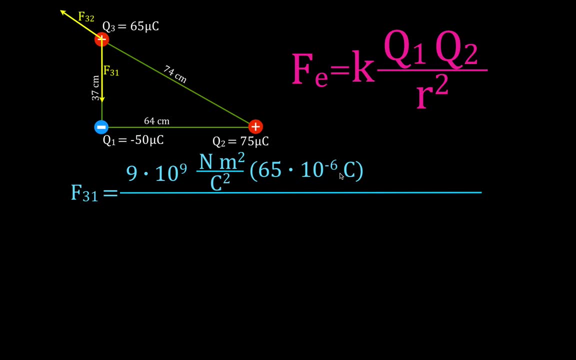 have to convert this to Coulomb's, because our unit isn't Coulomb's. We can't leave it in microcoulombs. Q2, now let's see that's Q1.. Now that's actually Q3.. Since I have F3 here, 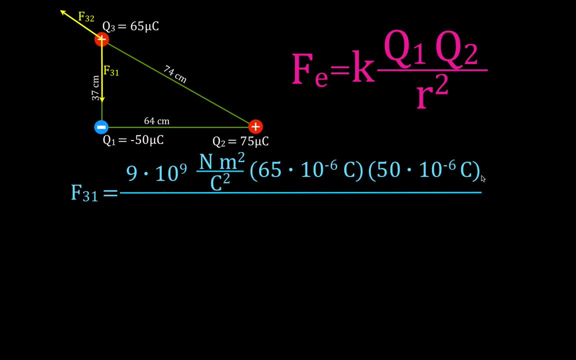 I put three first And then Q1 is 50 microcoulombs. You notice this is negative. we calculate the magnitude. We don't use the negative and the positive signs, so to speak. We don't use the negative signs. We determine the direction with whether the forces 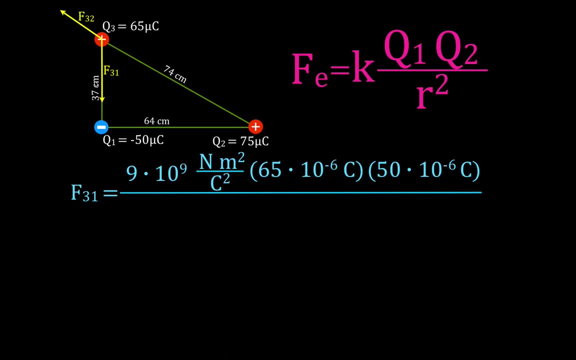 what do they call that? Repel or attract? Okay, and then we're going to square the distance between them. It's 0.73 meters. square that, and you get that the force on three from two acts in this direction and the magnitude of the force is 214 newtons. All right, 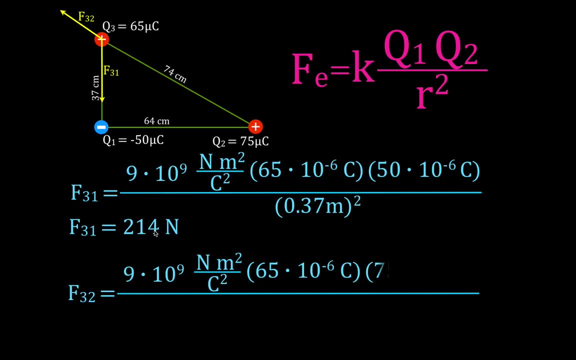 now let's do the same thing for 3,2, the force on three from two: Again Coulomb's law, Coulomb's constant: Again F3, 65 microcoulombs. This time F2 is 75 microcoulombs. 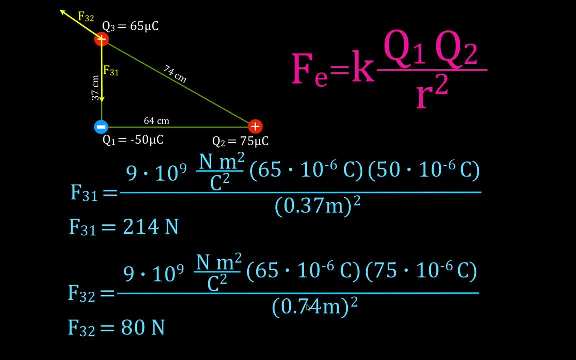 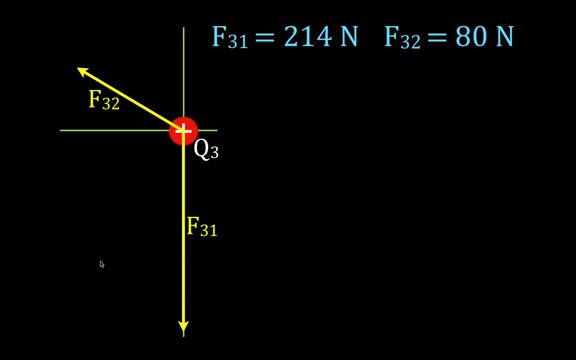 and the distance between them squared and you get that the force on three from two is 80 newtons. Okay, so now we know the direction and the magnitude of those two forces and we'll deal with that in the next slide. We know, as we figured out in the previous slide, F3,1 is 214. 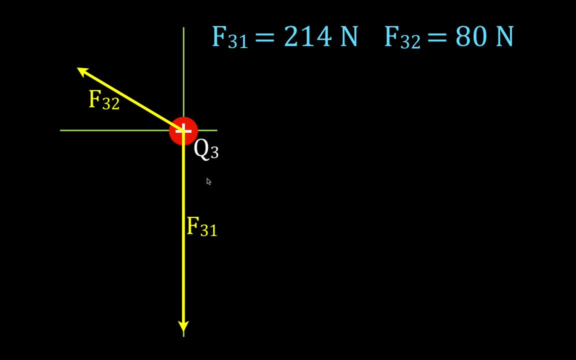 newtons is 80 newtons And I try to draw them a little bit to scale. This one is obviously longer than this one. This force is directly on the y-axis. This force is acting between the x and the y-axis. 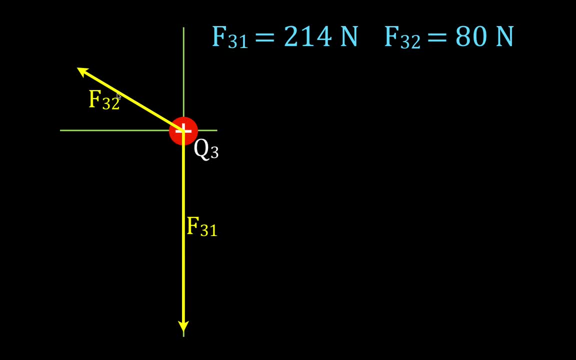 and that means we have to break this vector, decompose this vector into its x and y components. So this vector- F32, has a component in the y direction and it also has a component in the x direction, F32y and F32x, And we're going to use our trig functions to decompose this vector. 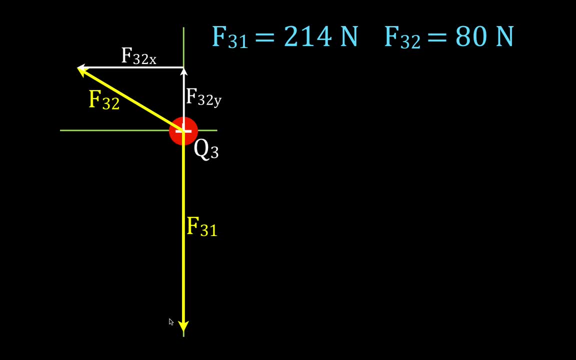 You should remember that we had a 30,, 60,, 90. We had a 60 degree, a 90 degree and a 30 degree. If this was 60 degrees, then that means that this angle right here is also 60 degrees. So you should. 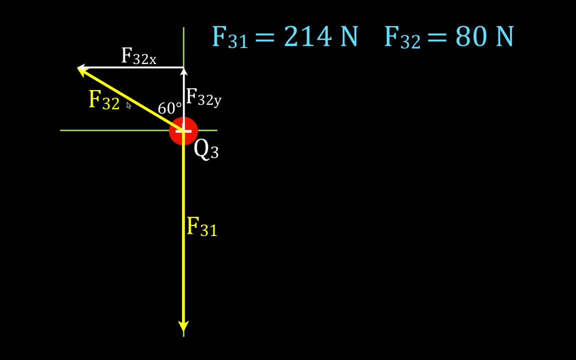 be a right triangle. We know one of the sides of a hypotenuse. We want to find out the other two sides. We know the angle trig F32x. F32x is on the opposite side of the angle, so we use the sine function And we get that F32x is. 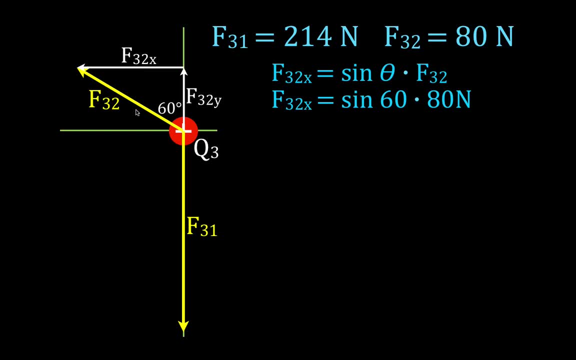 the sine of 60 degrees, times 80 newtons, times the hypotenuse, And we get that the length of that side is 69 newtons. Then we have F32y is the cosine, It's the adjacent side And the cosine. 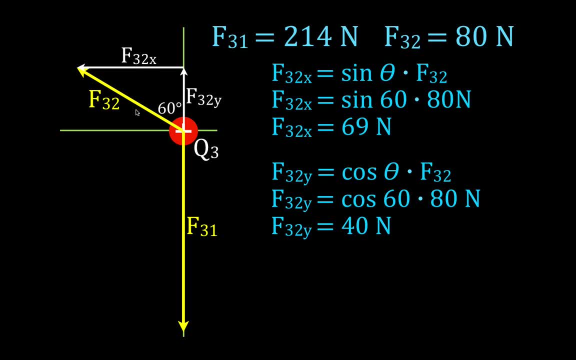 of 60 times 80 is 40 newtons. Now we know we only have one force acting in the x direction. The total force acting in the x direction is 69 newtons. We calculate that That's this force. But you'll notice now, in a sense we have two forces, that y component of 32 and 31 acting in. 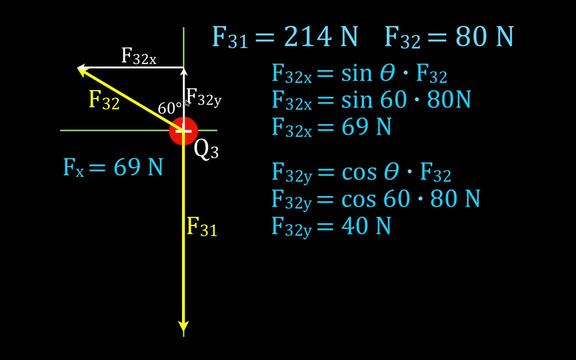 the y direction And they're acting in opposite directions. So we're going to add them up. in a sense, We're going to subtract 32y from 31. And we get that total force. the resultant force in the y direction is F31 minus F32.. And that gives us 214 newtons minus 40.. 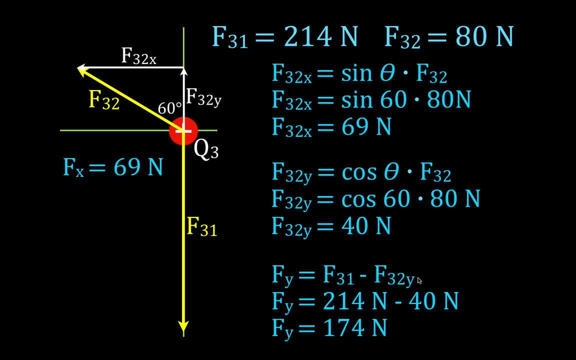 And that tells us that the total force acting in the y direction is 174 newtons. So now we really have our two forces, one in the x, one in the y direction- 69 newtons and the y direction 174 newtons, And now we can figure out the resultant force of those two. 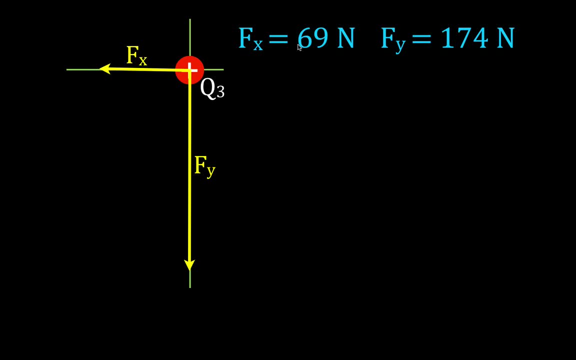 And here we have: the force in the x direction is 69.. The force in the y direction is 174.. I can add these two vectors up now, head to tail. Move the y one over And the resultant force- the net force acting on Q3, is simply represented by. 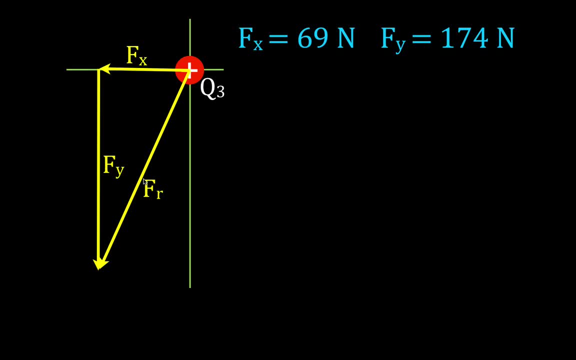 this vector. Now, once again, we have trig Pythagorean theorem. In this case, we know the two sides. We want to figure out the hypotenuse and the angle. So let's see what are we going to do first. Oh, this is the angle. I'm going to designate this as the angle theta. And, in order, 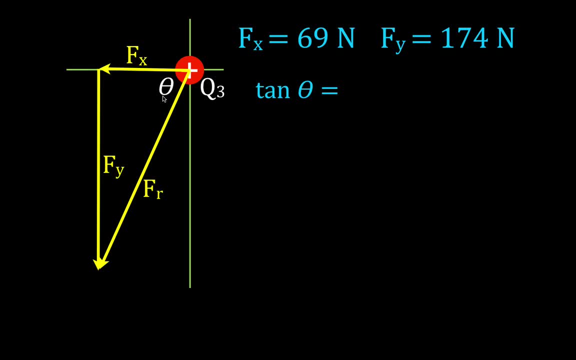 to find the angle. I'm going to use the tangent because I know the tangent is the opposite. over the adjacent, The opposite is the opposite. So I'm going to use the tangent because I know the y, The adjacent is Fx. I'm going to divide Fy by Fx. Fy is 174.. Fx is 69. Divide that, I get the. 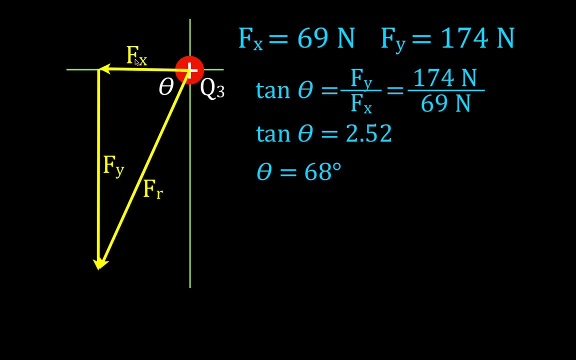 tangent of the angle is 252.. I have to take the inverse tangent, I get theta. This angle right here is 68 degrees. So this angle is 68 degrees. If you start with this x-axis as 0, you go all. 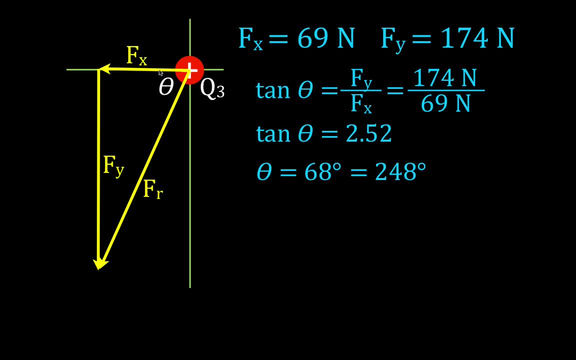 the way around, It's 180 plus that and you get 248 degrees. So the direction of the force is in that direction, either 60 to 80 degrees, So the angle is 80 degrees below the negative x-axis or 248 degrees from the positive You count. 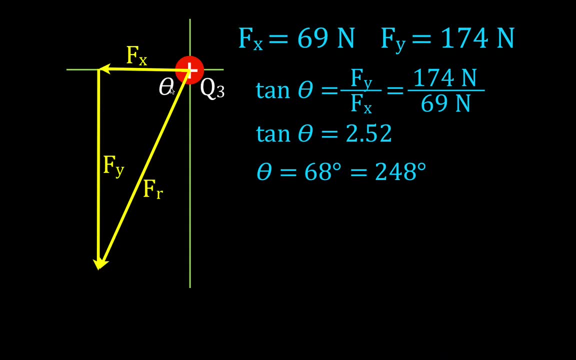 this way, counterclockwise. Third quadrant: Okay, now we need to find out the length of this side, or the length of the hypotenuse, or the magnitude of the force. It's really just a triangle. We're going to use the Pythagorean theorem: c squared equals a squared plus b squared. We want.